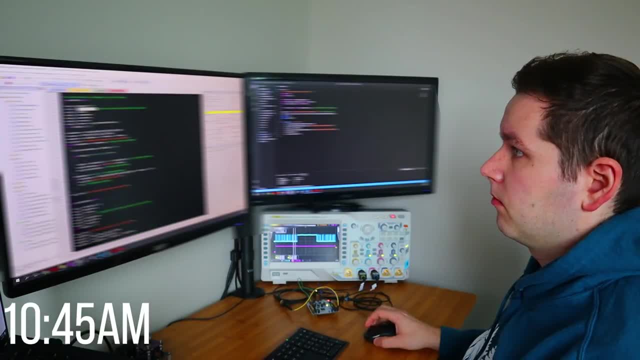 with butter or something like that. Next up, I continue working on my Jira tasks. Unfortunately, I can't discuss a lot of details about the work I'm currently doing due to the nature of my job, but I will try to show you as much as I can. So today I'm working with an STM32. 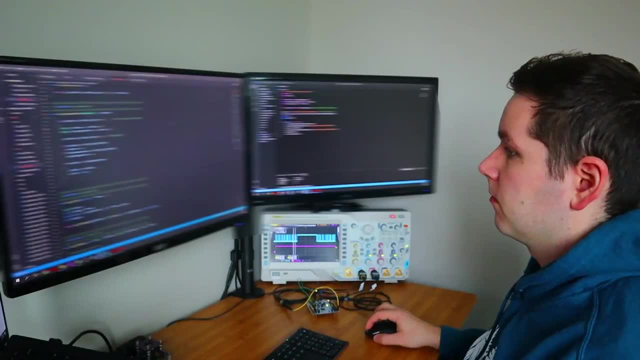 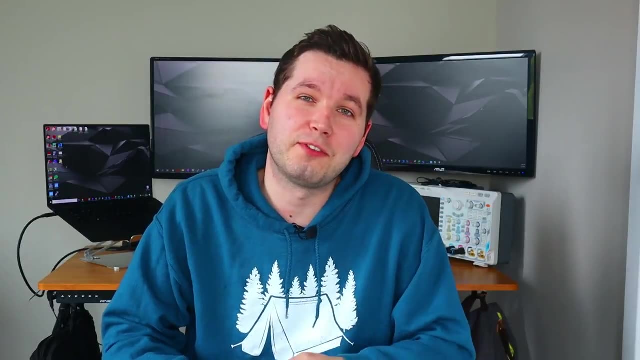 nuclear board that runs a free RTOS operating system And today I'm using it to test out some communication code via USB for actual prototype board. It's very common for embedded software engineers to use an oscilloscope or a signal generator to help debug their code. Today 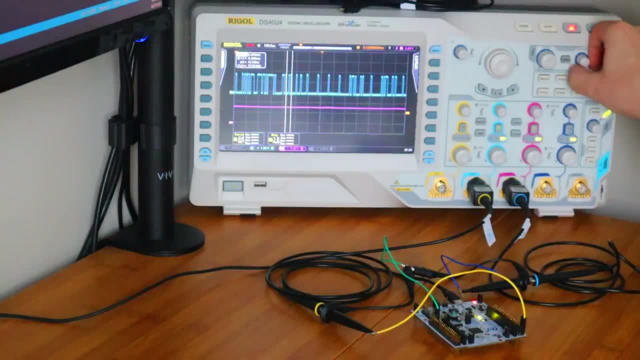 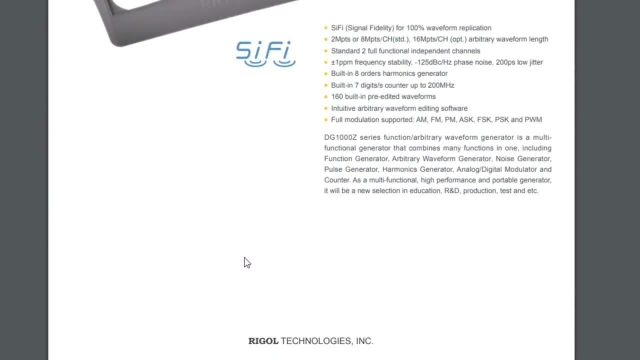 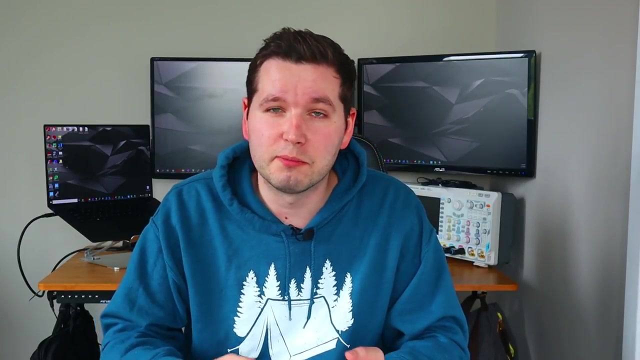 I'm using the oscilloscope to make sure data sent via peripherals is correct and works in general. There are also cases when we would use a signal generator on these development boards to simulate signals from sensors that we might use Because embedded software. engineers work with the hardware and the software. it is important for. 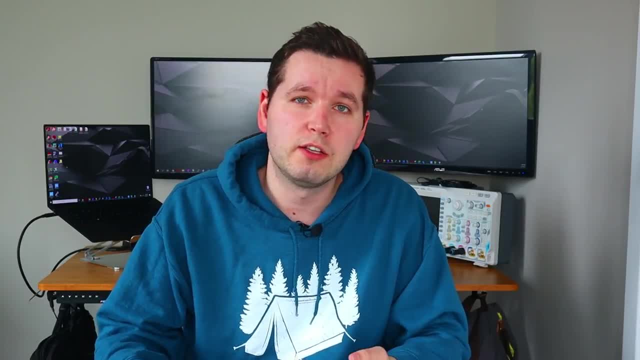 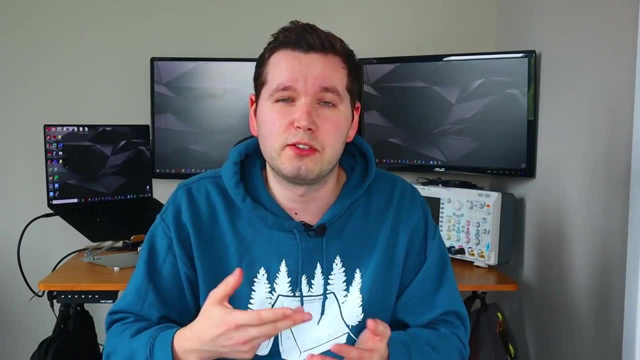 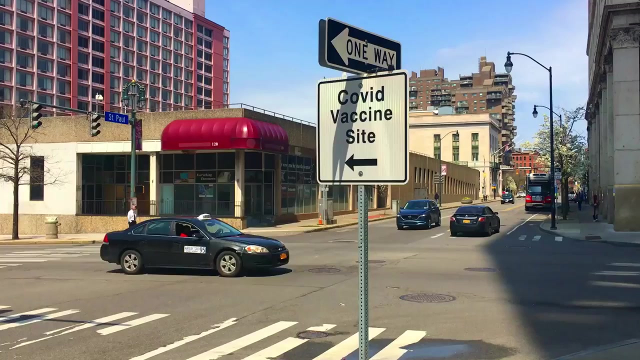 them to understand both aspects of the development phase. So they would need to know about how to read electrical schematics, but also how to write the software, how to write clean code and do all that electrical components work properly with the software. Today I'm actually getting my second. 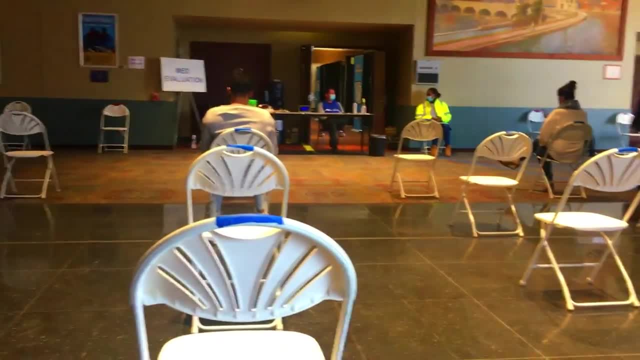 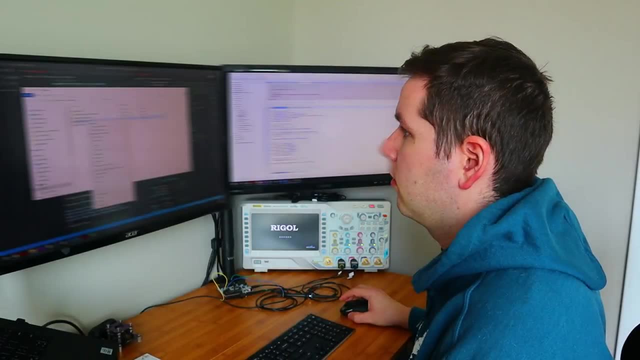 COVID shot. So thankfully, my employer lets us take some time off for doctor's appointments, which is great. After that, I just keep working on my code and other tasks that I might have. One of my code reviews got approved, So now it was time for me to go ahead and merge this code. 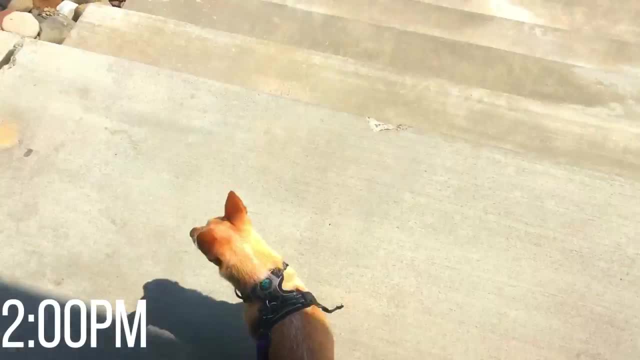 from the branch to the trunk. Around 2 and 3 pm I take another 15-minute break to take my dog out for a walk. Usually during that 15-minute break I still keep thinking about what I'm going to do, So 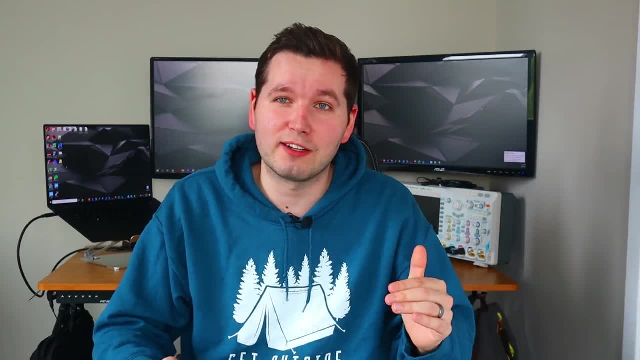 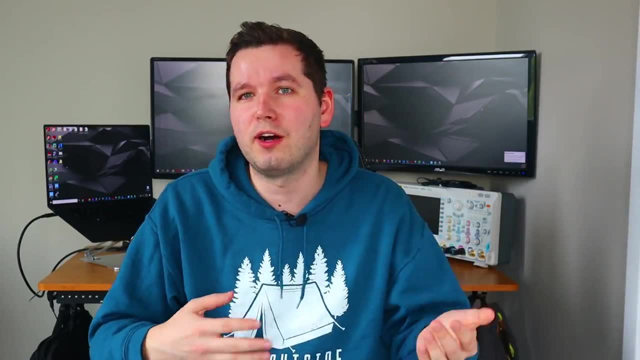 I'm thinking about work. I think about the stuff that I've been working on. If I'm stuck on something, it's a great time for me to take my eyes off of the computer and just like clear my mind outside, walk it out and maybe come up with a good idea that might solve the issue that I'm 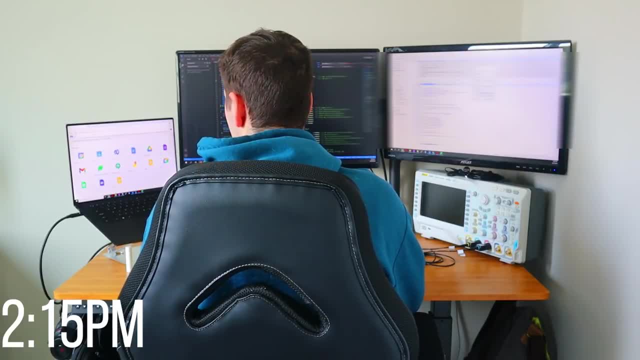 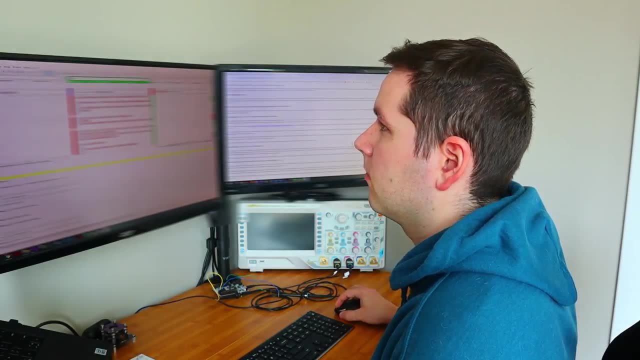 facing currently And right after that, I keep going with my code and debugging. During this process, apparently something went wrong and my code wasn't passing my test cases that I wanted it to pass, And so I had to figure out what's going on, And after a few hours I was able to.